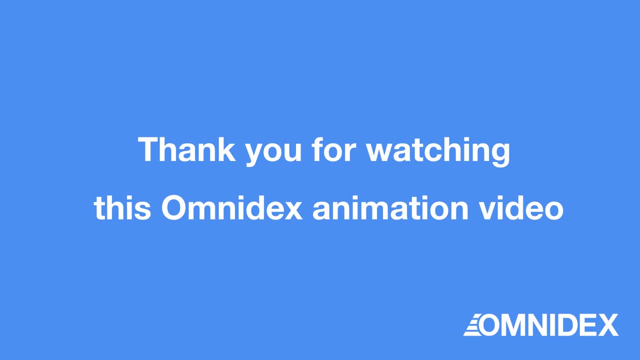 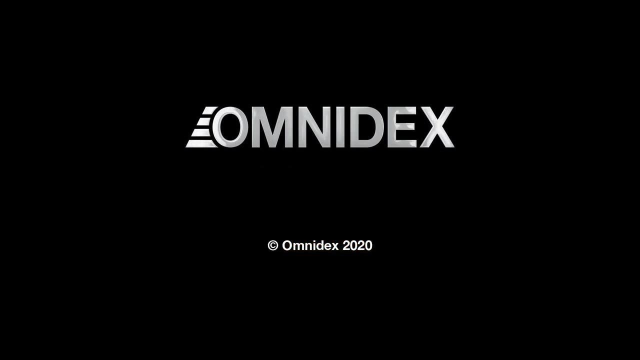 Thank you for watching. Check out other casting processes on our channel. If you have any questions or other problems, please post them in the comment section. 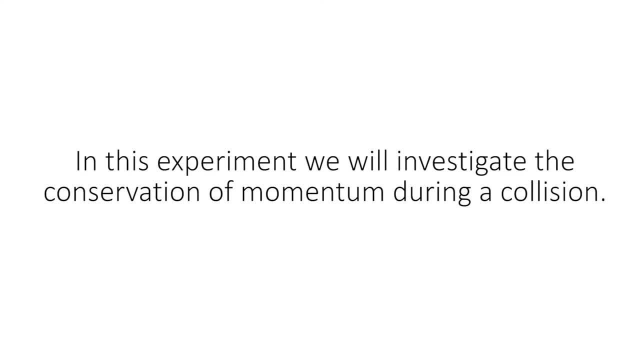 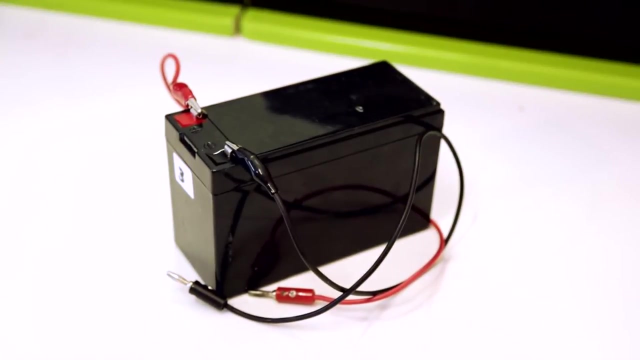 Conservation of momentum. In this experiment we will investigate the conservation of momentum during a collision. The apparatus: a dynamics trolley, a rail track, a ticker timer, a mass piece of known mass ticker tape and a 12 volt battery with leads. The method: set up the trolley. 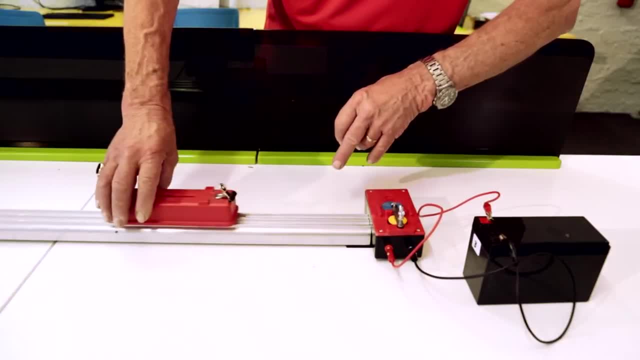 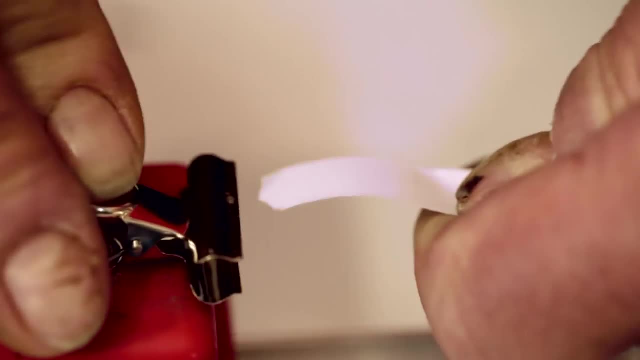 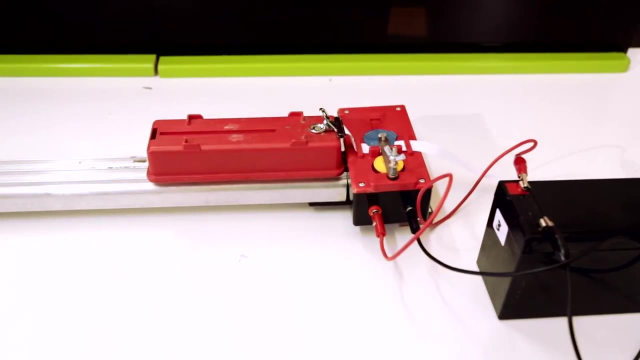 of known mass capital M on the rail. Feed a length of ticker tape through the timer and attach it to the rear end of the trolley. The timer has been set at 40 hertz. This will give 40 dots per second. Hold a mass piece of known mass small m midway above the rail, allowing 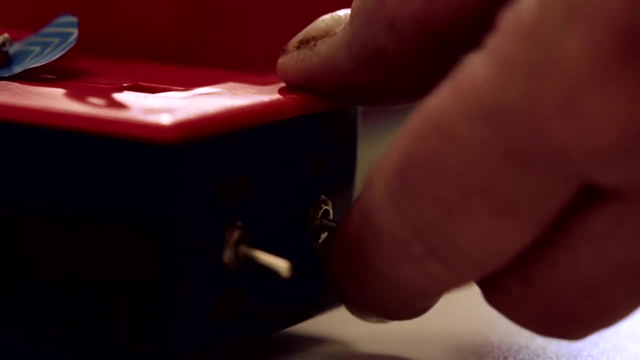 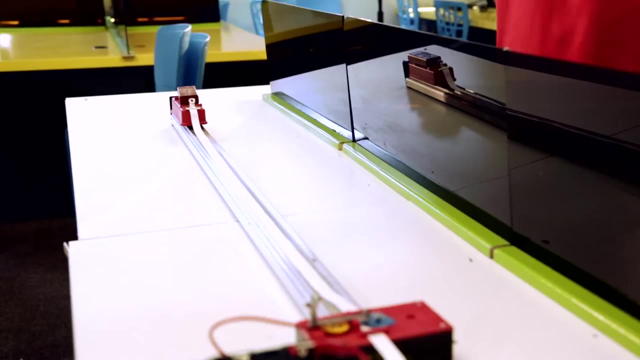 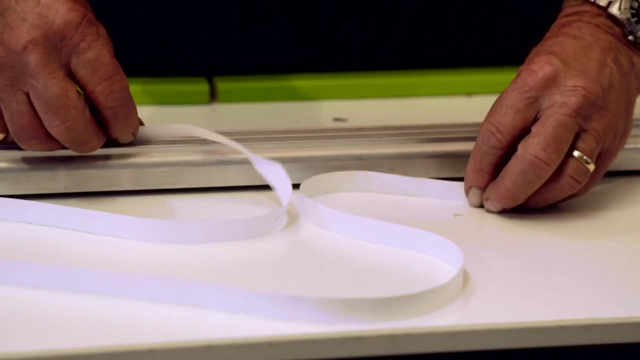 the trolley to pass underneath it. Switch on the timer and give the trolley a gentle thud Thrust, sufficient to let it run the full length of the trolley. When the trolley is below the mass piece, let the mass piece fall onto the trolley. When the run is complete, remove the 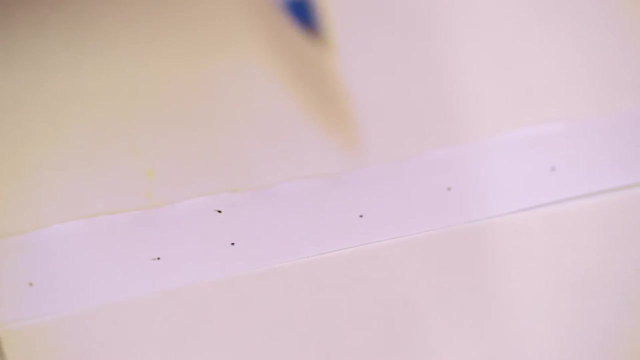 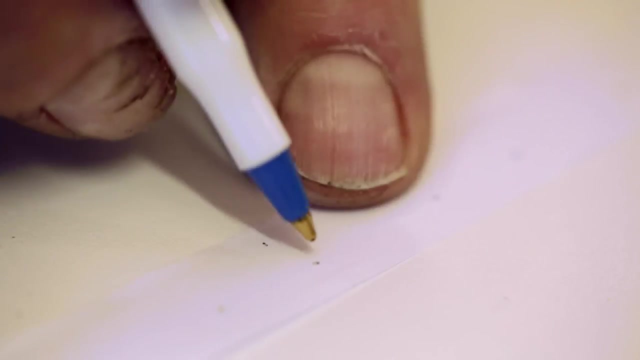 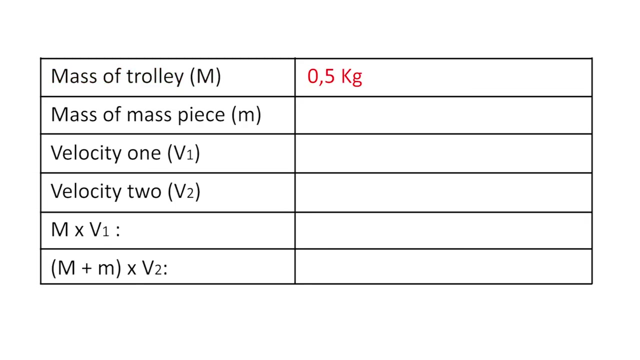 tape and calculate the velocity of the trolley before and after the collision. Remember that velocity is equal to the displacement divided by the time. The distance between 10 dots is covered in a quarter of a second. The mass of the trolley, capital M, was 0,5 kilograms. 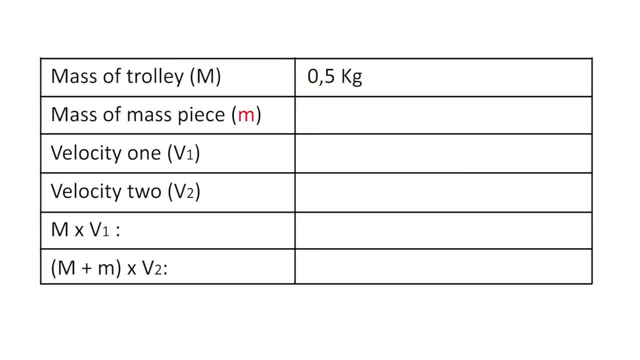 The mass of the mass piece: small m, 0,25 kilograms. The velocity before collision was 0.38 meters per second. The velocity after collision was 0,240 secondes per second. The mass of the trolley was by 86,000 green championship batteries In the last temperature controlled.